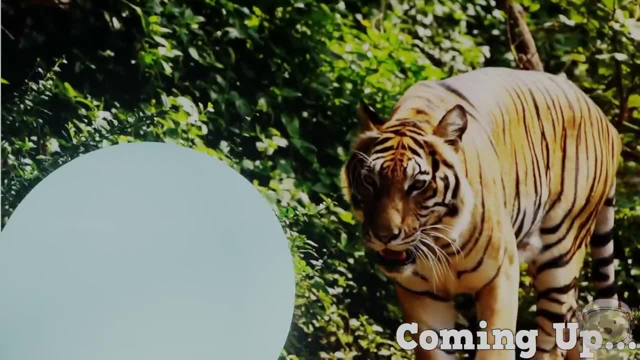 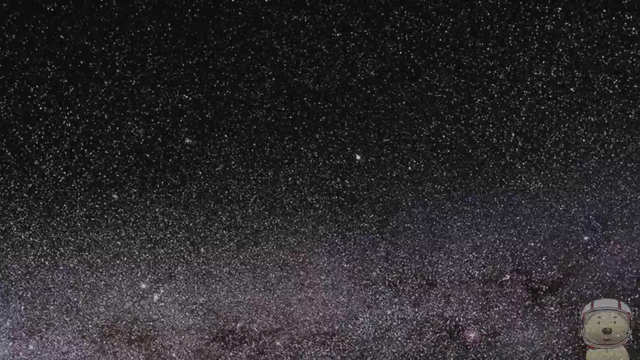 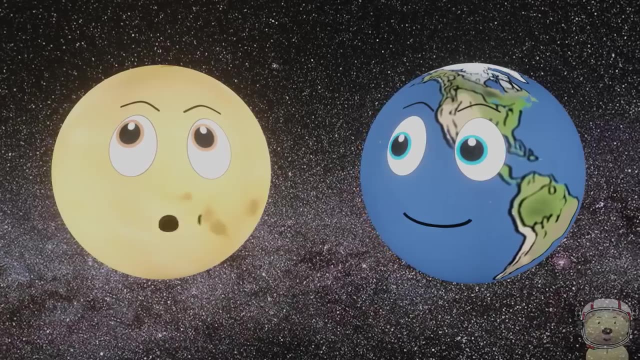 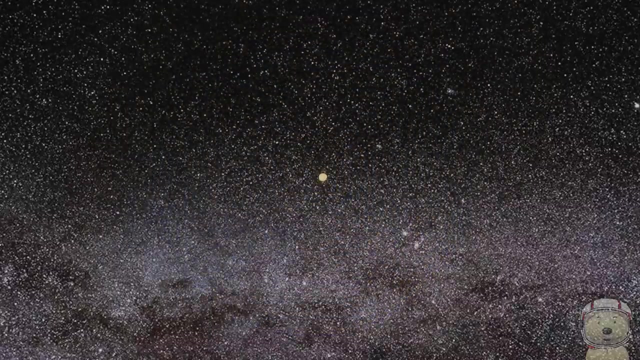 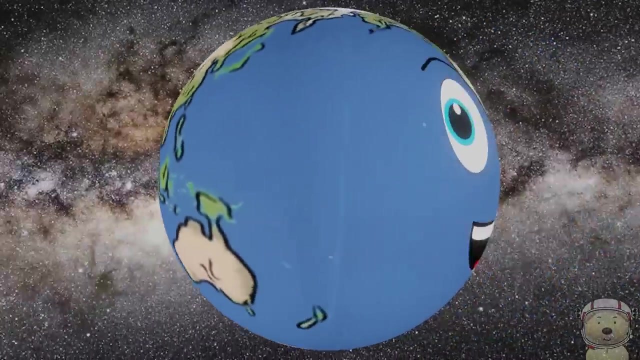 Coming up, Uh, Okay, okay, guys. What are we going to learn about today, then? How fabulous I am. No Venus. Today we need to shrink down and visit one of my rainforests. Apparently, the size of rainforests is decreasing each year, and we need to find out why. 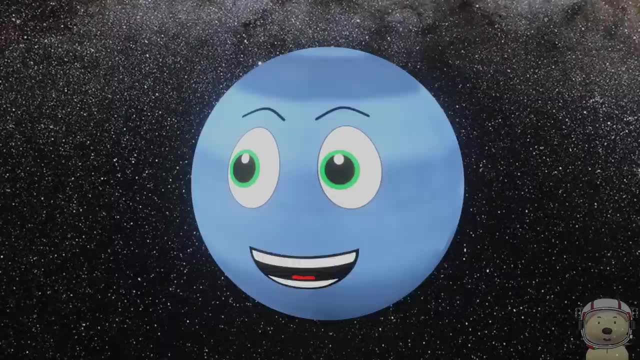 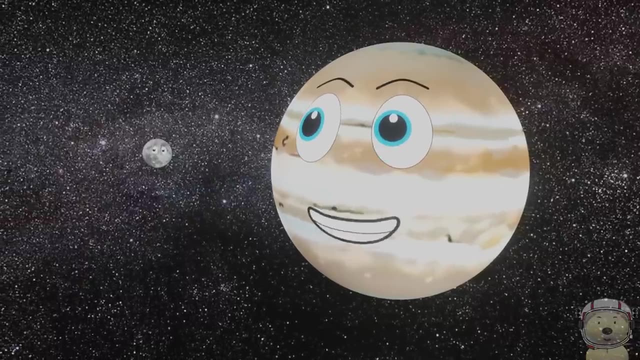 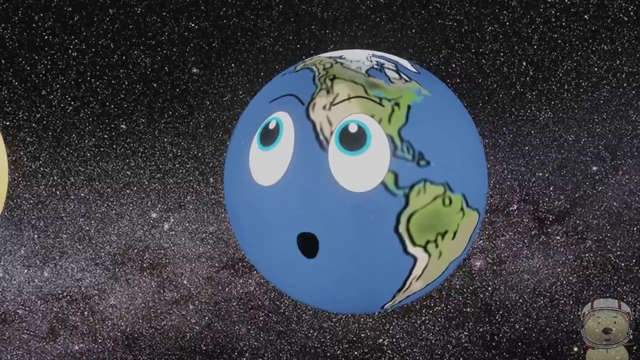 Is that the jungle? Yes, sometimes Rainforest is the correct name, but you can call it a jungle too, Merc, and I will stay and sort the video link. Who is going Well? me, Venus, Neptune, Mars, Saturn and Uranus. 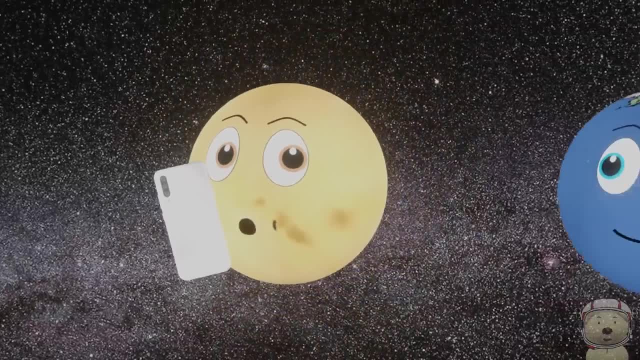 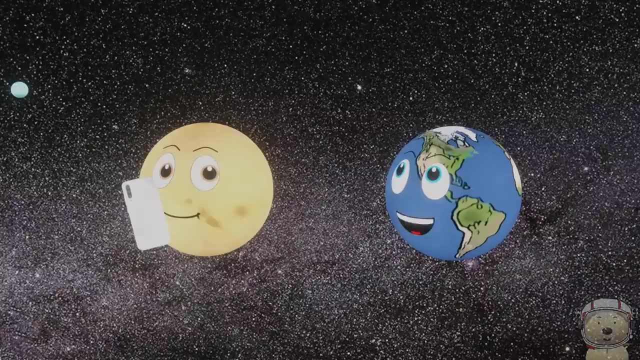 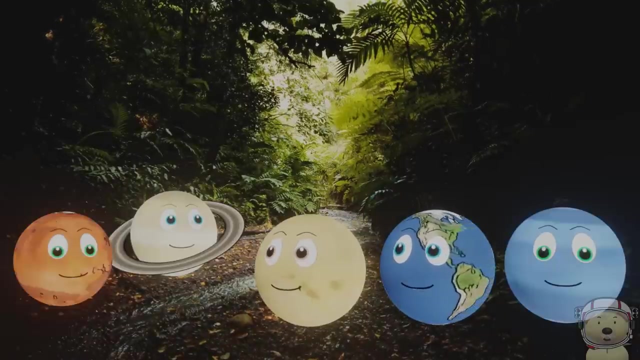 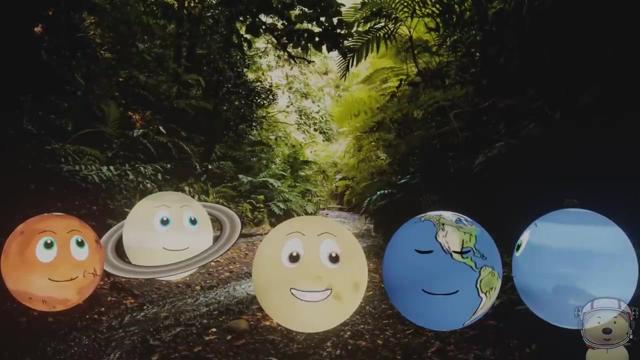 But Uranus is late. We can wait no more Shrinking down. Hello, wait for me. Quick, hurry up, Uranus. Okay, Uranus was in the distance so he wouldn't have transported properly. He does this every time. We'll need to find him. 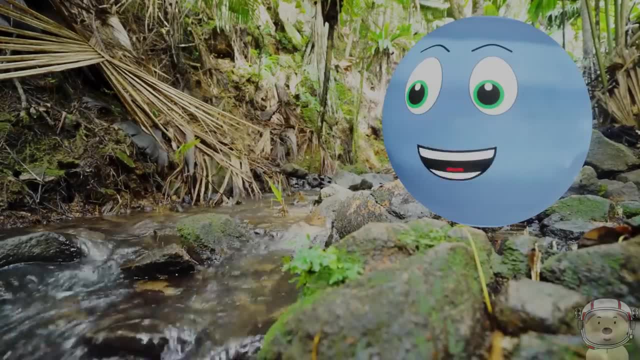 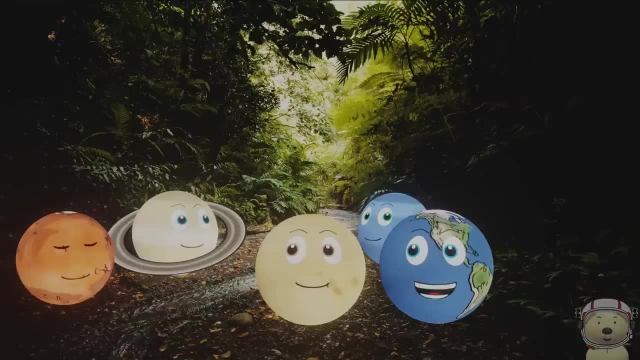 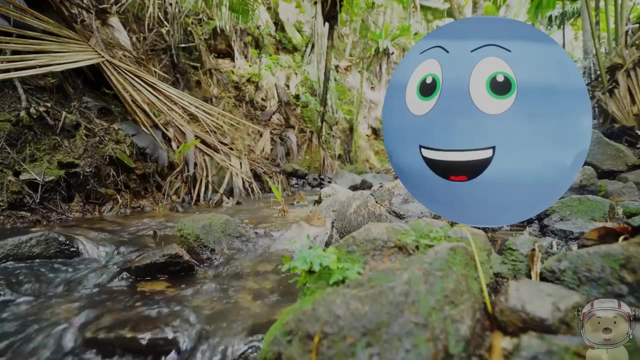 Okay, let's split up Venus and Earth. You go to the river together. Check along there. Great Stuck with Earth. Sorry, I'll have luck with Earth. Right, I'm on to you. Mars, Saturn and myself will check through the trees of the rainforest. 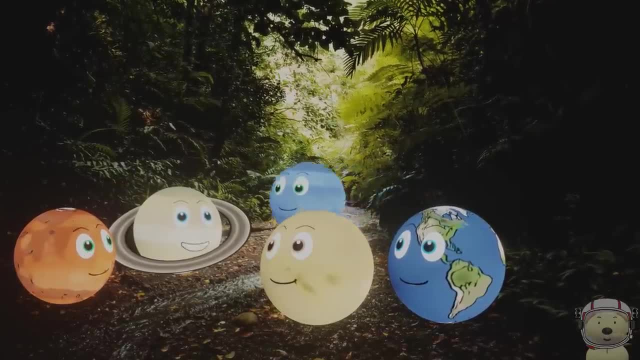 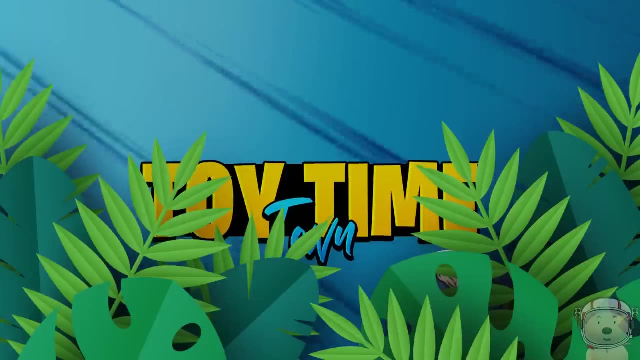 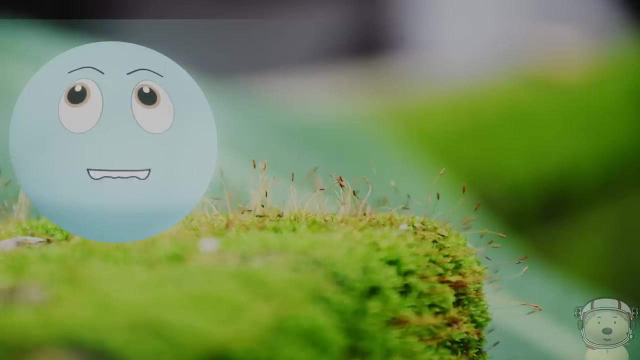 Don't forget dudes. We need to work out why the rainforest is shrinking Well, and find planet Uranus. of course, We need to find a way to get to it. We need to find a way to get to it. My, my Everything looks so big around here. 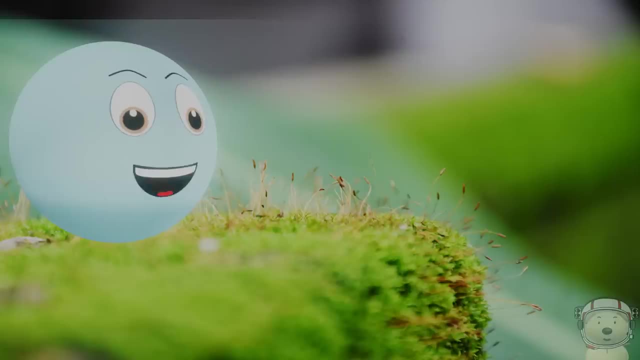 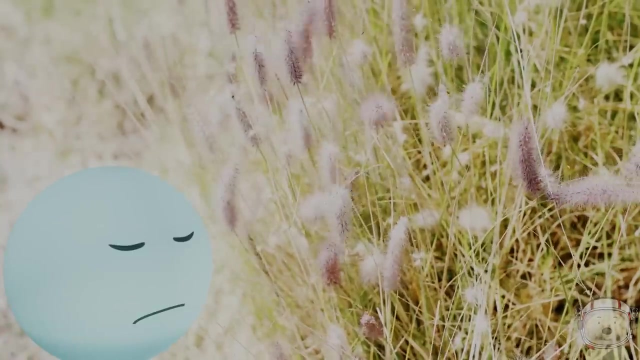 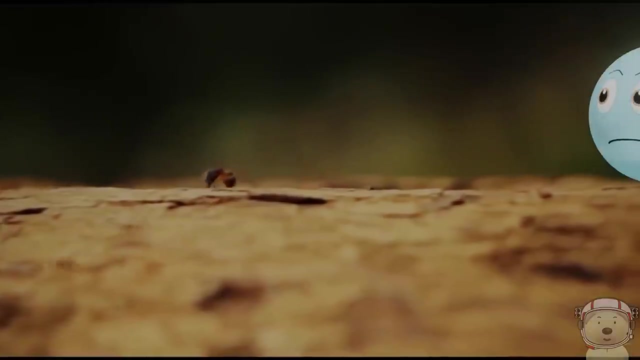 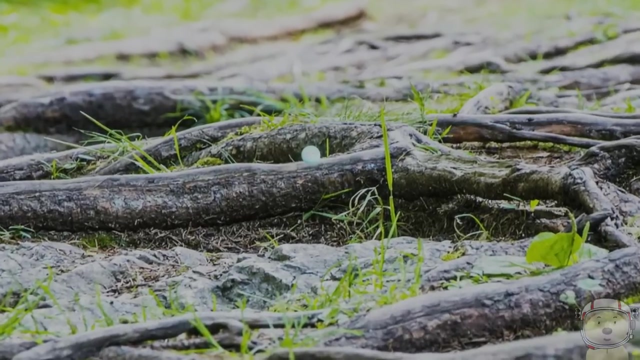 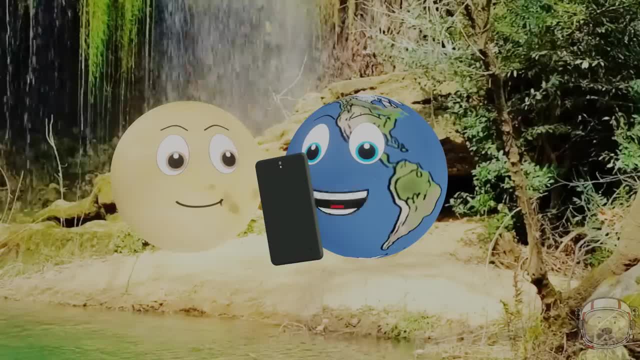 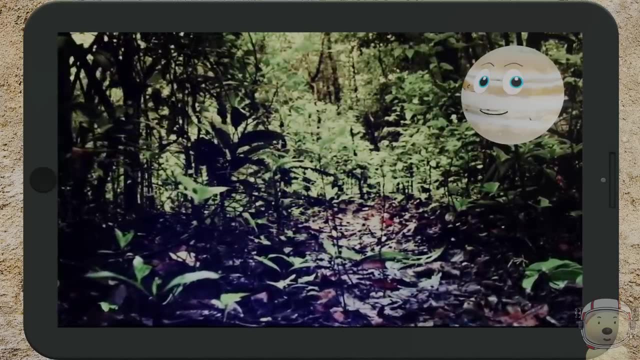 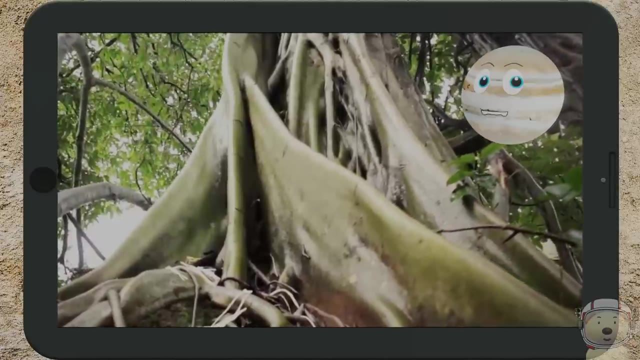 Okay, Venus, Here's the river Jupiter. what can you tell us about the river please? Hey guys, You are in a rainforest. in Asia, A rainforest is a tall, dense forest that receive lots of rain every year. 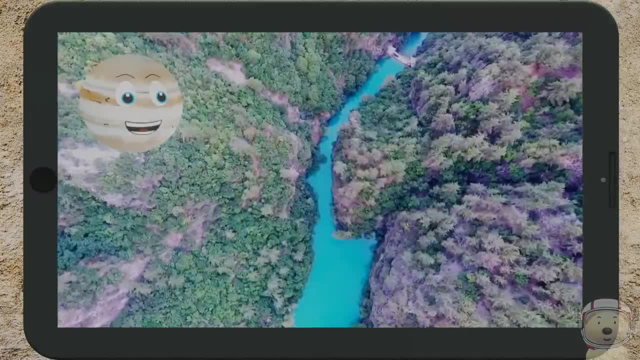 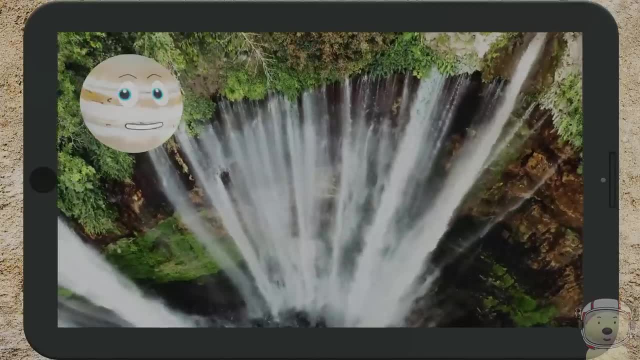 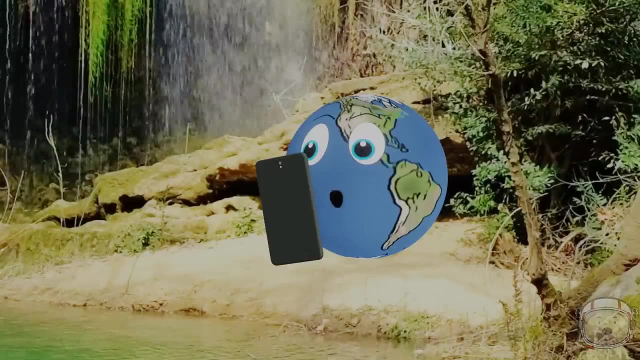 And with the amount of rainfall that rainforest gets, you need to be very careful, And with the amount of rainfall that rainforest gets, you need to be very careful. Thanks, Jupiter. Maybe we should be careful then. Maybe we should be careful then. 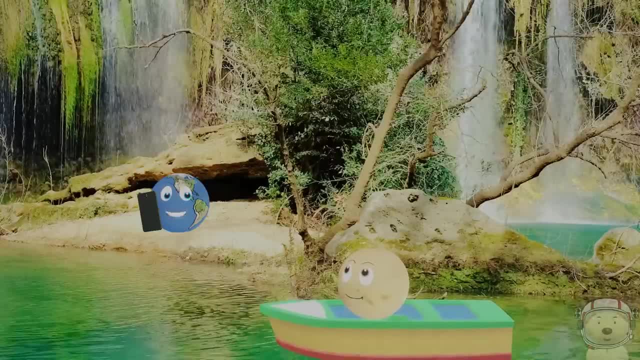 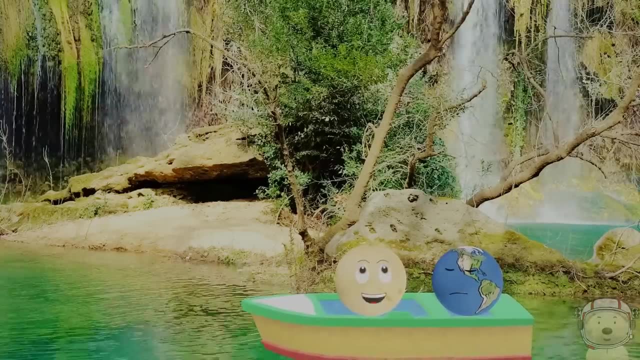 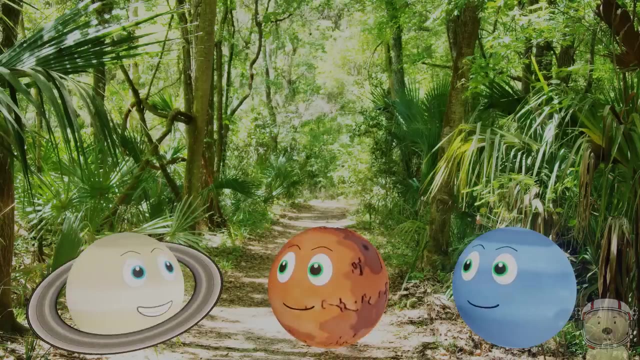 I found a boat, Earth Hop in. Maybe we should stay on land then. Maybe we should stay on land then. Yikes, I'm in Change of heart, eh, Okay, Okay, Look at these trees, dudes. That is a lot. 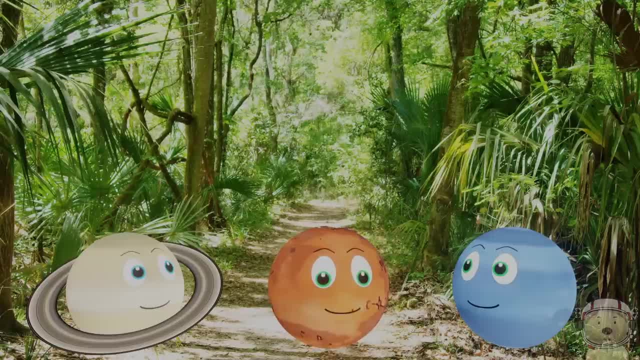 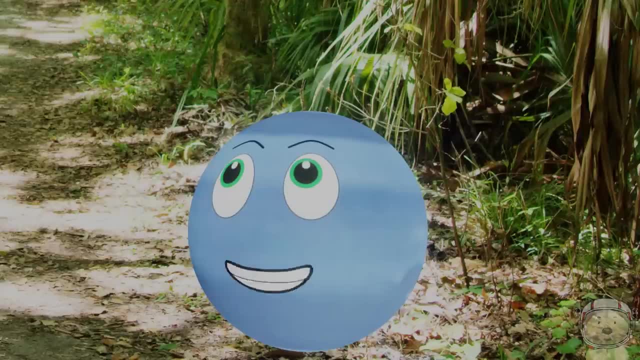 How are we meant to find planet Uranus? How are we meant to find planet Uranus? Maybe I could do a rap until he appears. Maybe I could do a rap until he appears. No, Maz, I think we need a better plan. 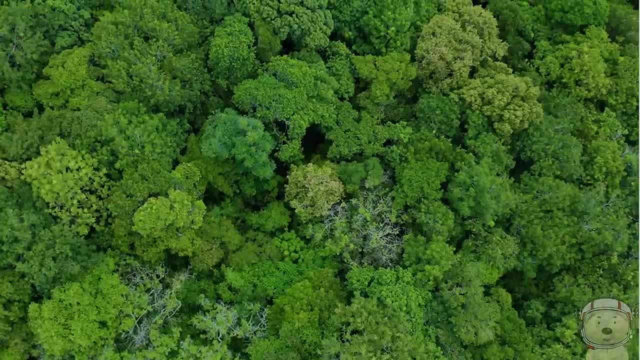 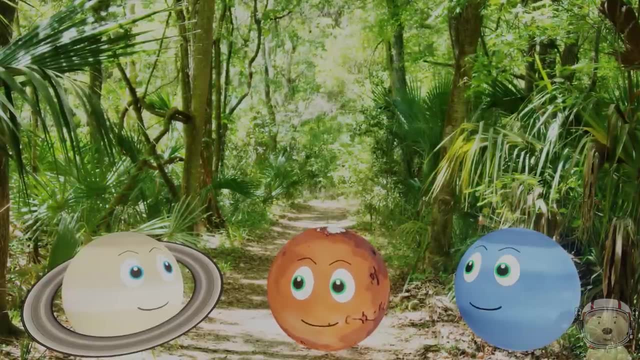 We should start by working our way into the rainforest. We should start by working our way into the rainforest, But jungle is massive. But jungle is massive, Right dude. We've got to start somewhere though, Behind Neptune. Oh, thanks. 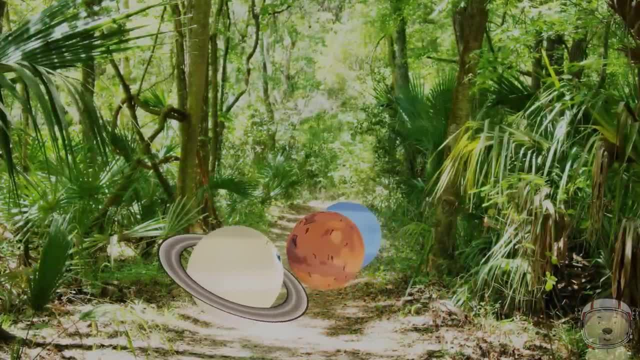 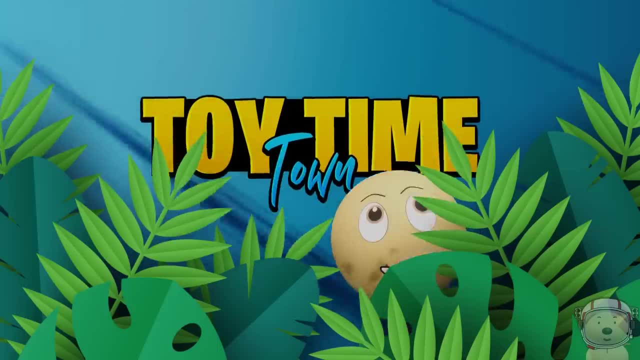 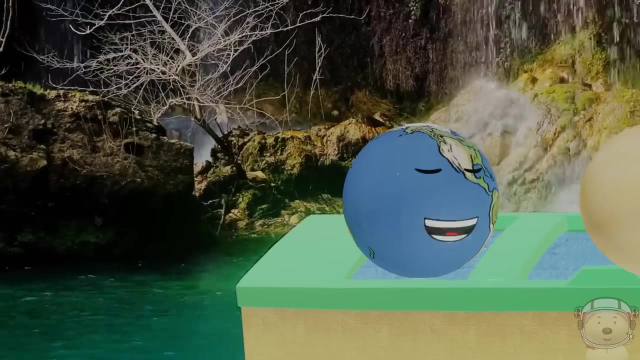 You have the rings. Maybe you should go first. What's my rings got to do with it? What's my rings got to do with it? Jungle is massive. I'm so hungry. Do you want pizza on you? Yes, Venus. 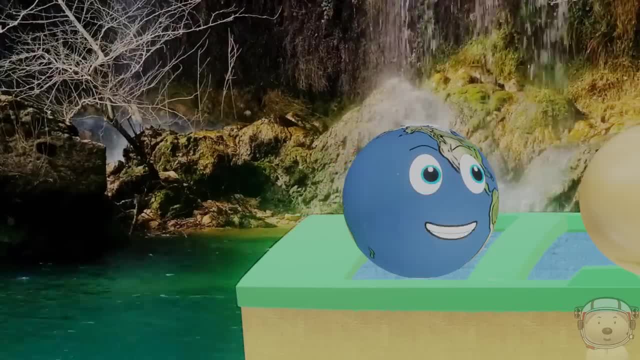 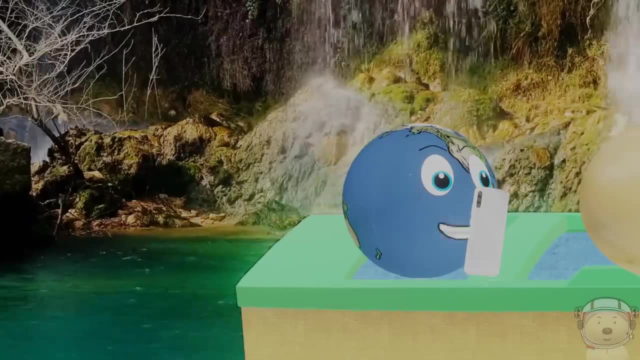 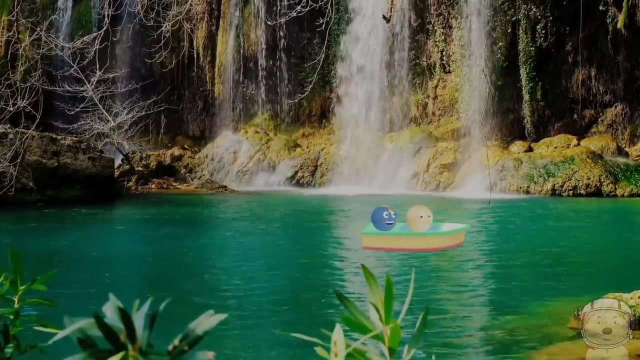 I always carry pizza on me, Just in case, Dear me, Good thing I do, then. Uh, I just got a text from Jupiter. Uranus is tiny By moving away when shrinking. By moving away when shrinking, he's been made even smaller. 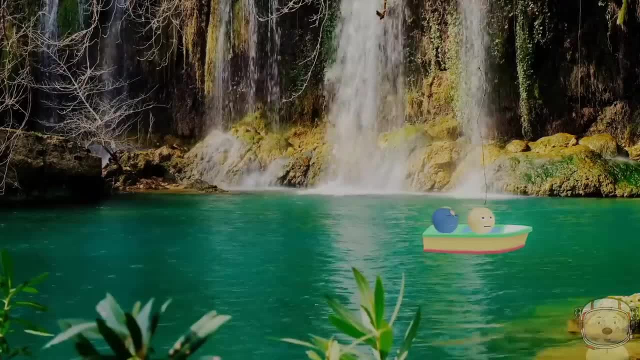 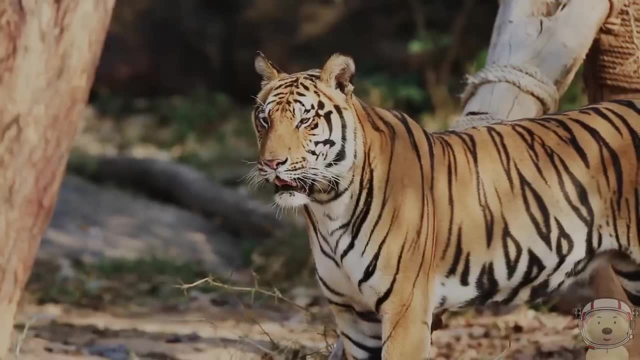 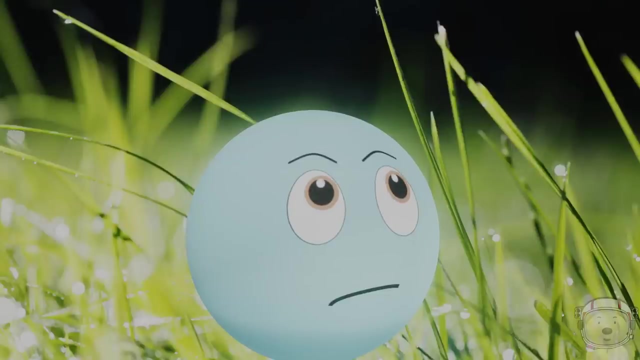 he's been made even smaller, So if we make him big again, we should find him easier. Yes, Oh no. Look there's a tiger over there. Look there's a tiger over there. Wow, A scary beast. 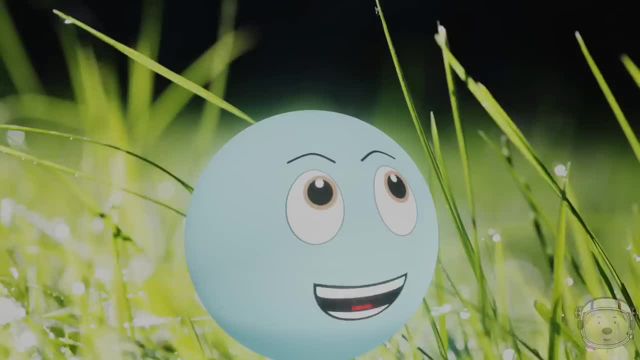 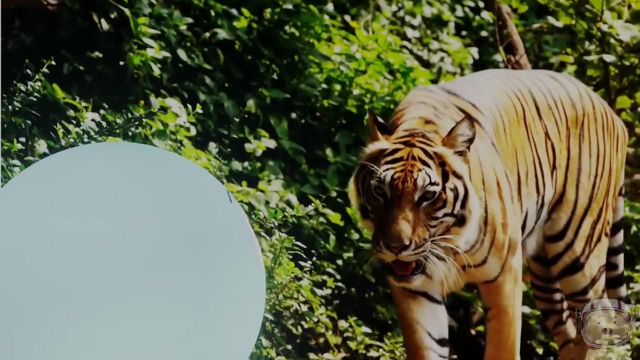 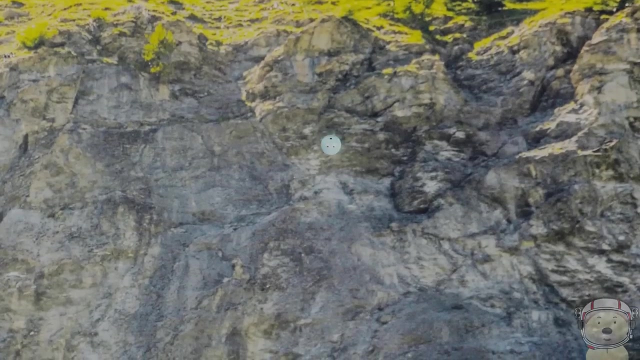 But he doesn't know I'm here yet. So as long as I stay small and hidden, as long as I stay small and hidden, that can't be good. Uh, Uh, Good kitty, Good kitty, Whoa, Okay, Venus. 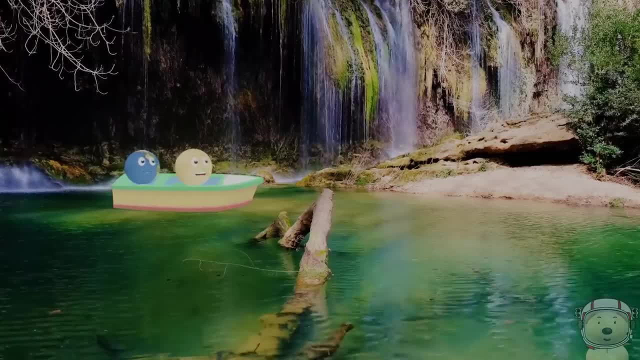 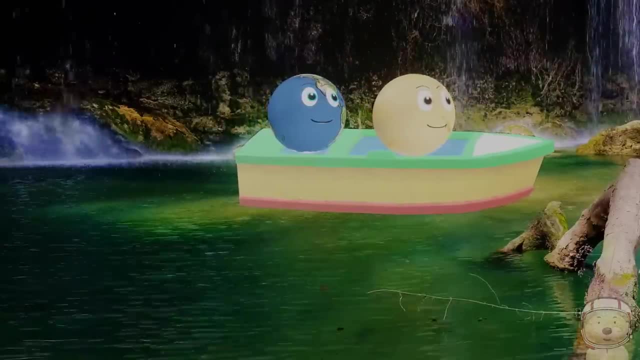 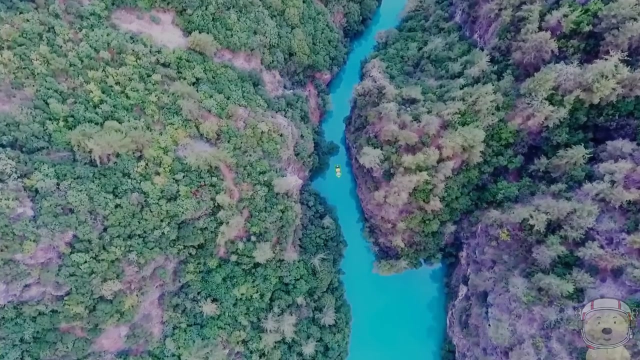 What do we do now? Hold on Three, two, one, Whoa, Whoa, Whoa. Okay, right, Get him in the boat. Right, Uranus, Stay with us this time. yes, Yes, but. 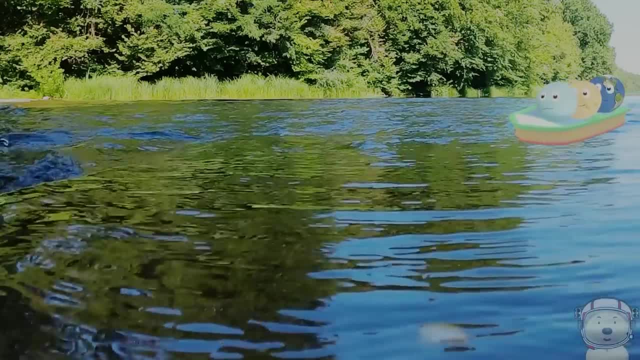 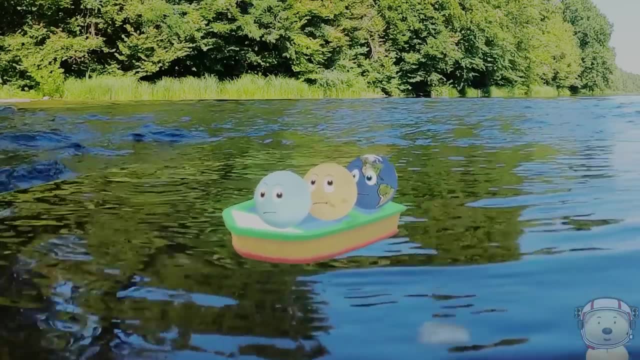 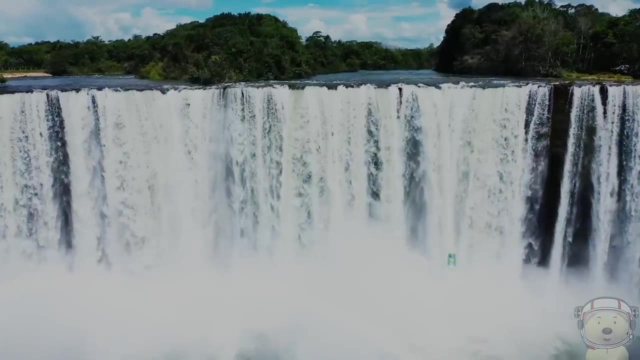 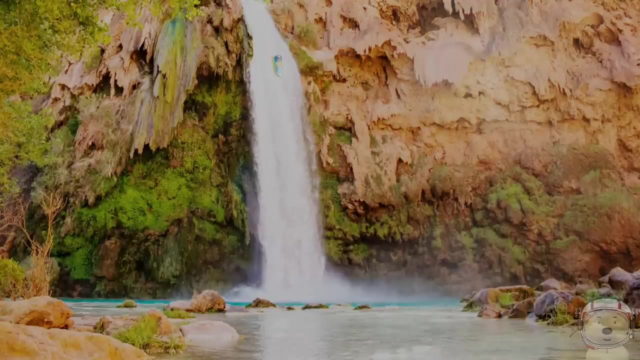 No buts Uranus. We need to stick together, I know, but But what Is that roaring noise? Uh, Uh, Whoa, Whoa, Whoa, Whoa, Whoa, Whoa, Whoa. 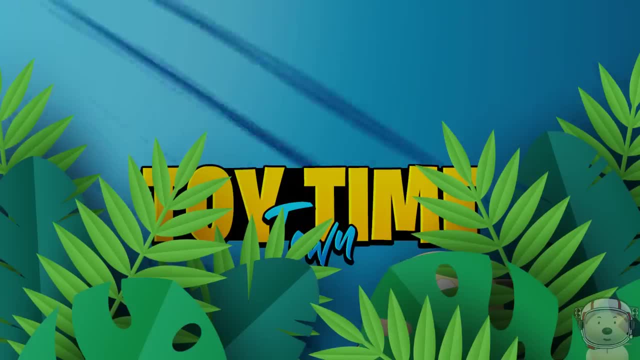 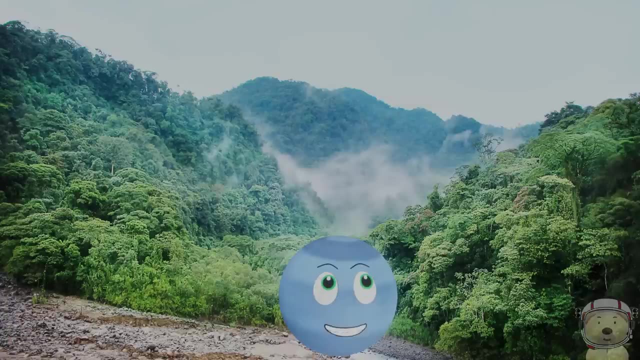 Can somebody else rescue me next time? Can somebody else rescue me next time? Okay, Uranus is safe. Okay, Uranus is safe. Any sign of why the rain forest is shrinking? Any sign of why the rain forest is shrinking? Nope. 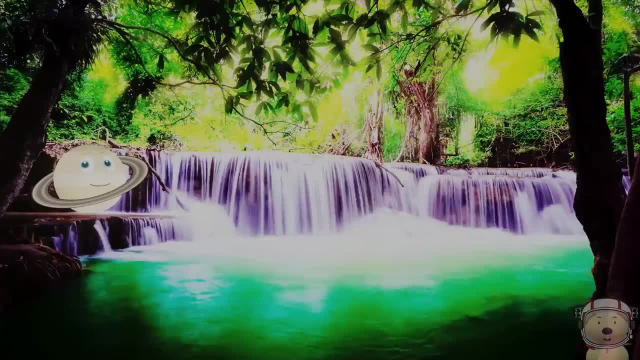 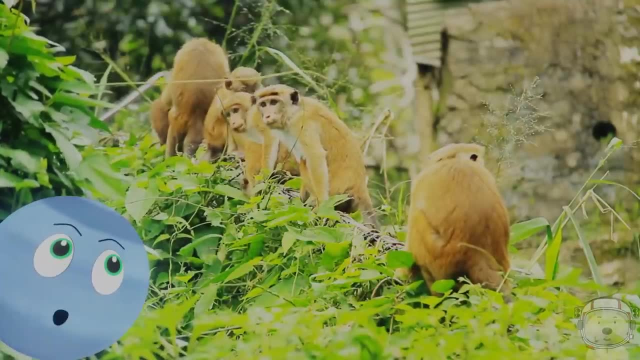 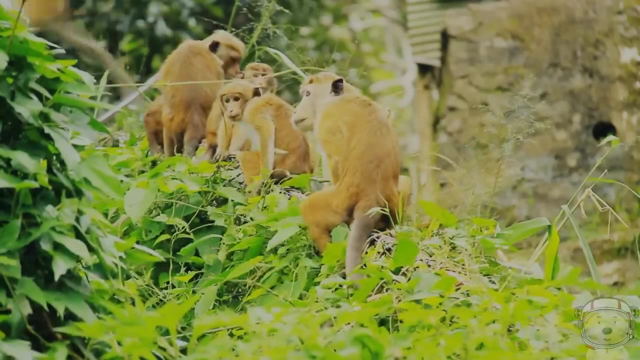 All good here. Nope, All good here. Nope, All good here. No, All seems good here. No, All seems good here. Hi guys, All good here. then Make sure you keep your eyes peeled. Brilliant, Brilliant. What is this? 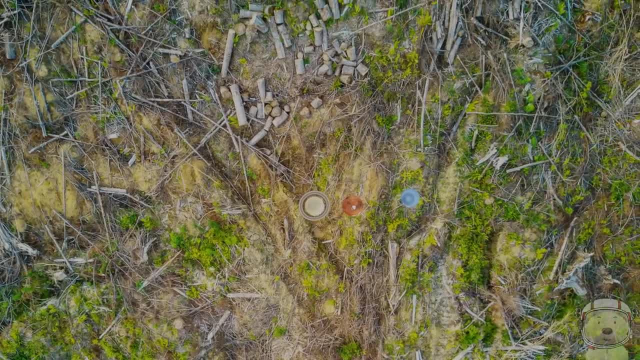 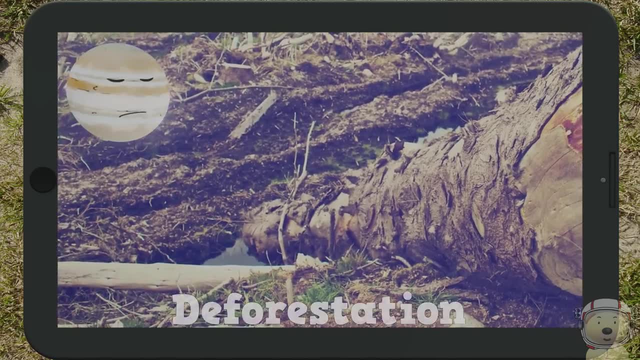 What is this? Where have all the trees gone? Jupiter? is this the cause of the Jupiter? is this the cause of the Jupiter? is this the cause of the rainforest shrinking? Yes, Deforestation means the removal of trees.